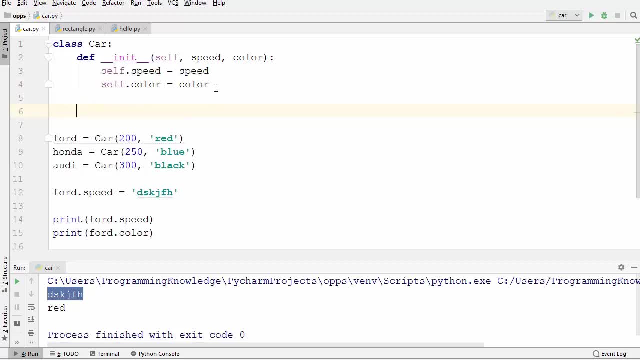 our code, we create functions. So let's create our first function, which is to set the value of speed. So I'm going to just say set underscore speed and inside the parenthesis it's going to take self as the first argument, which is the default, and second is the value of speed. So I can say value here, right, and then, once we have the value of speed, we can just call self dot speed. 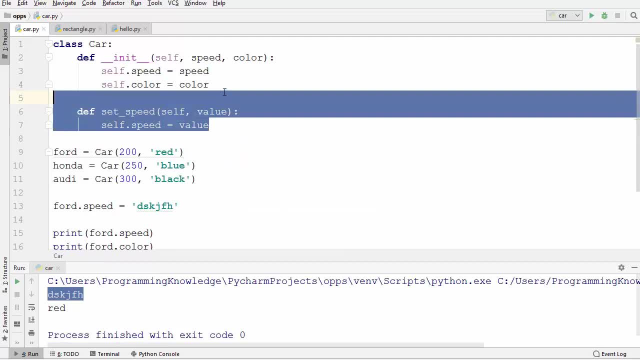 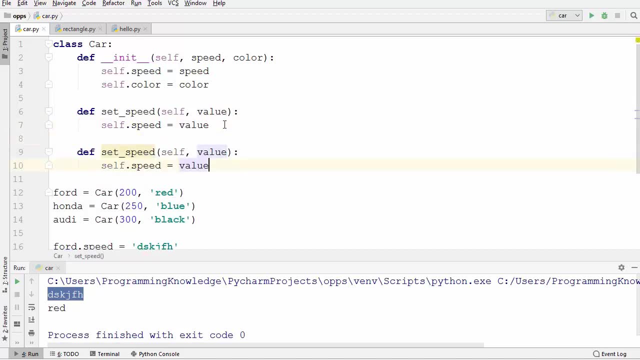 So let's say, self dot speed is equal to value. Similarly, we can create a get method for the speed. So right now we have created the set method to set the speed and now we are going to create a get method to get the speed. and in order to get the speed, we don't need to pass any argument, we just need to return the speed which is already set. So we can just write return and then self dot speed. So we have 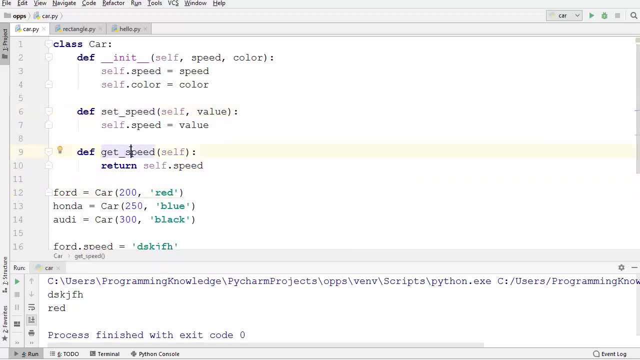 created two functions: set and get. These are also called setter and getter for the attribute, which is speed in our case. So let's use these functions instead of this kind of setting of data. So first of all, I'm going to call this forward object dot set speed method out of this object and then I'm going to pass the new speed using this set method Now, in order to get the speed I can write instead of this forward object dot set speed. 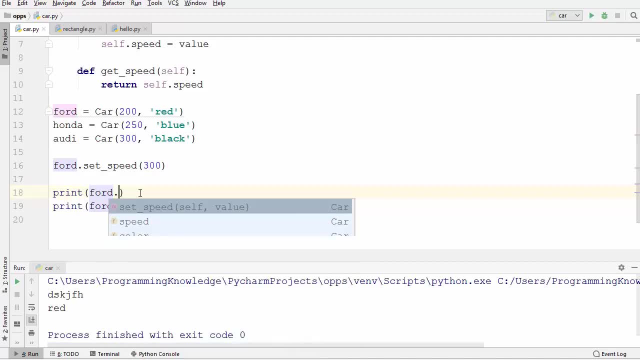 dot speed. I can just write the Ford dot get speed, which is going to give me the speed of this Ford object. so I'm going to run the code and you can see it prints the speed which we have set using the set method, but still will this. 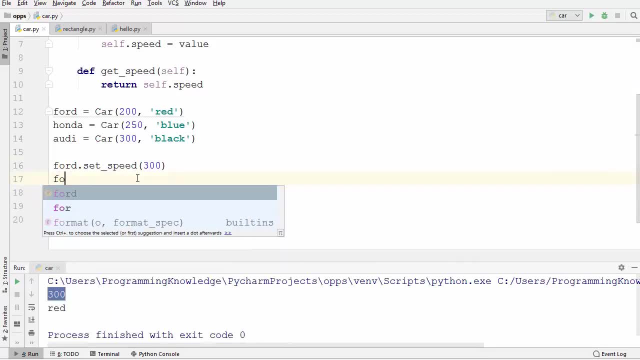 protect your data. let's see. so I'm going to once again try to use Ford dot speed and then I will try to set the new value of speed. will it be a problem? no, so you can see, when I try to get the speed, the new speed is set, and we want to prevent. 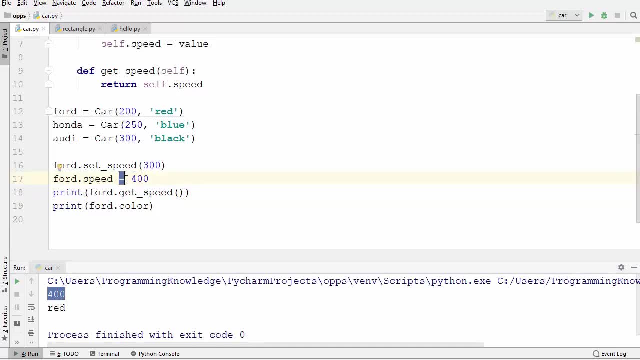 this kind of setting of data. using this equals to symbol, so we need to somehow make our attribute private. now, if you are familiar with other object oriented programming languages like Java or C++, they use the keywords like public, private or protected in order to mark their attributes or the member variables as the private, or public or protected. 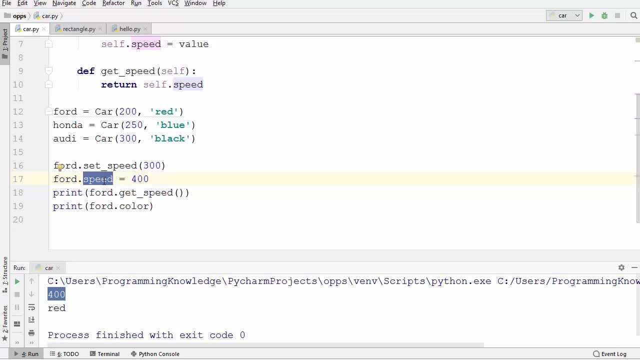 but Python doesn't have any of these keywords. so how we can make our data private? so let me give you first of all an example. so I'm going to go to this class, which is hello, and here I'm going to set some values. so first value: 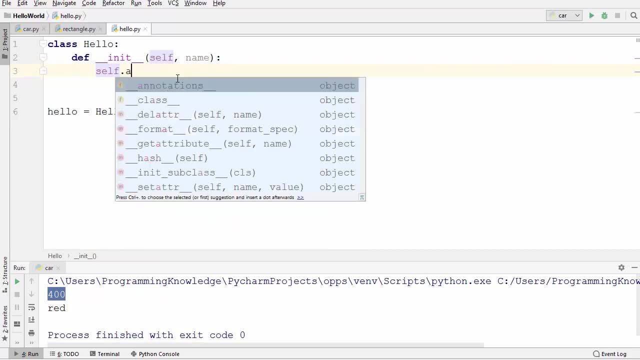 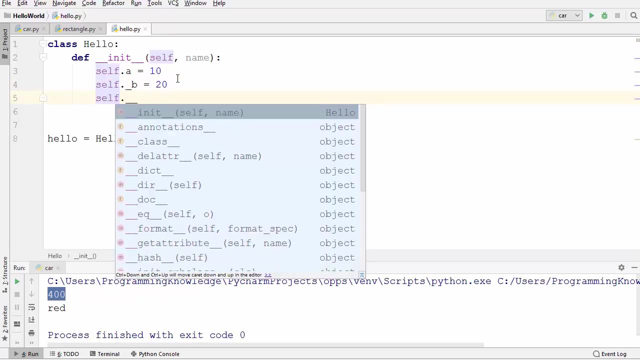 is, for example, self dot a is equal to 10. second value is self dot underscore B is equal to 20 and the third value as self dot underscore underscore C is equal to 30. so we have created three member variables in this hello class. one is a. 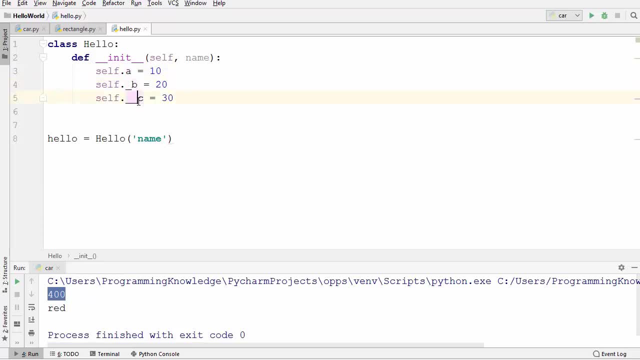 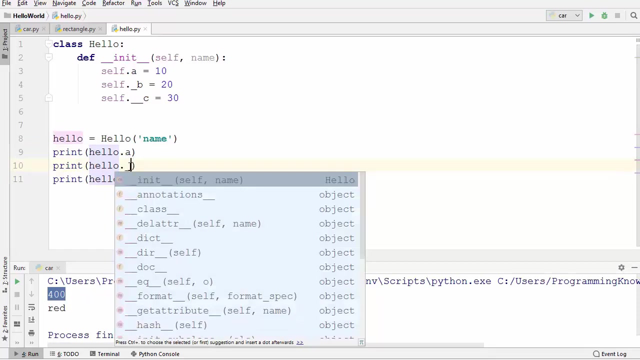 second is underscore B and the C is with two underscores in front of it and let's try to access all these three values. so I'm going to just use the print method and then the hello object, dot a, and similarly I will use this print to get the value of dot underscore B and also. 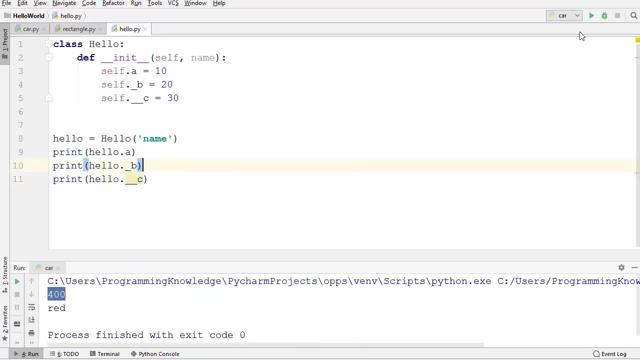 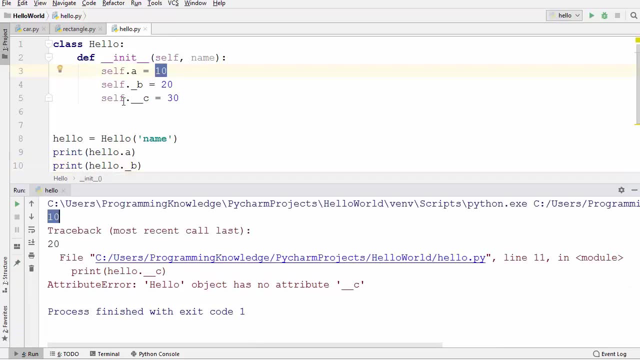 dot, underscore, underscore C, and let's try to run this program and let's see what happens. so let's try to run this program and let's see what happens. so let's try to run this program and let's see what happens. and you can see here: the first value which is printed here is 10, which is the. 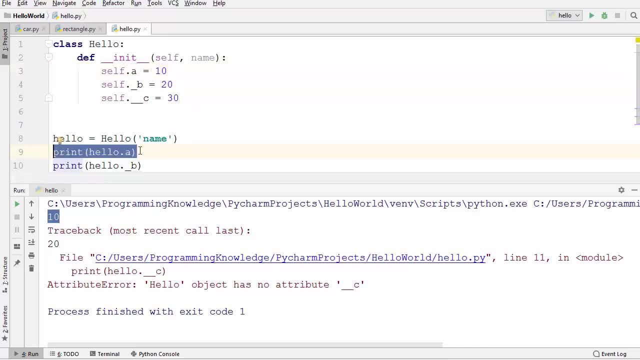 value inside the a variable. so this code was executed successfully. now we can see here that 20 is also printed. that means this code is also executed successfully. but at the time of underscore, underscore C. when we want to use this underscore, underscore C outside the class, it says: hello, object has no. 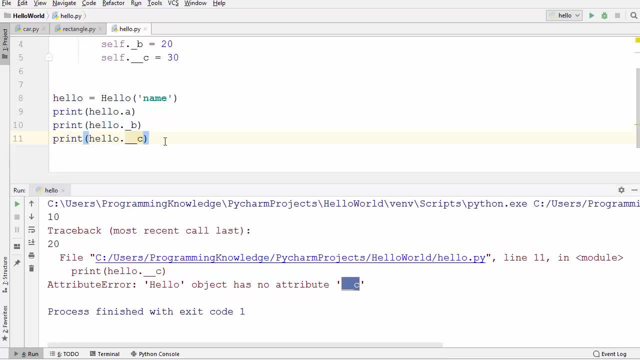 attribute called underscore, underscore C, and this is the point. so underscore, underscore- you can use to make your attribute private. okay, so this is a convention. there is no keywords like private in Python. that's why Python uses this kind of convention in which whenever you use double, underscores it. 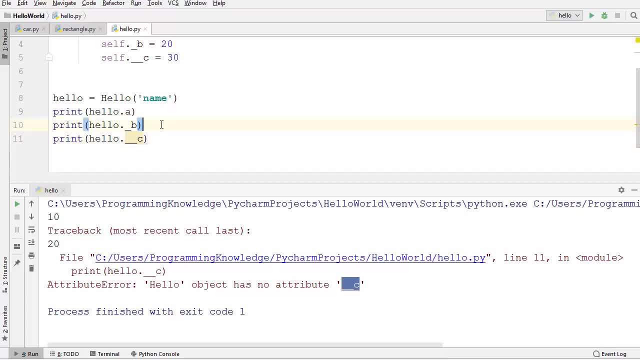 makes your data private. when you use single underscore, that also means that it's a private variable, but this is only a convention. nothing stops you to change the value of underscore B or accessing the value of underscore B. okay, so if you truly want to make your data private, then use double underscore in front of your. 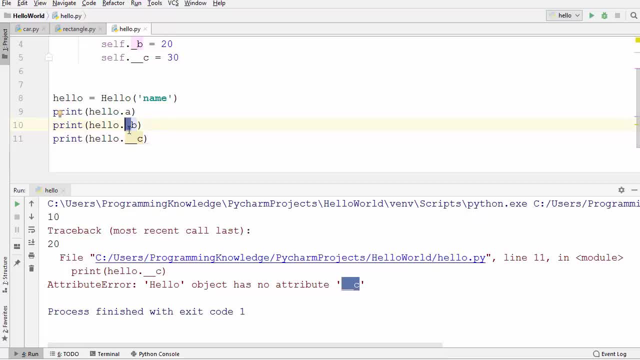 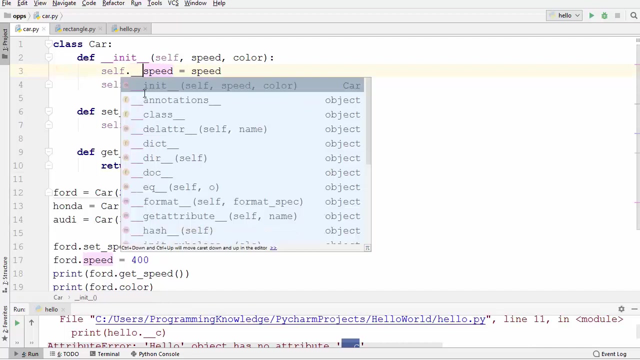 variable. when you use single underscore, that means it's a partially private variable and it's only a convention. okay, so let's go to our car class once again. and now we know that we can add double underscore in front of our variable name. so we have two variables here. one is speed, so let's add double list underscore. 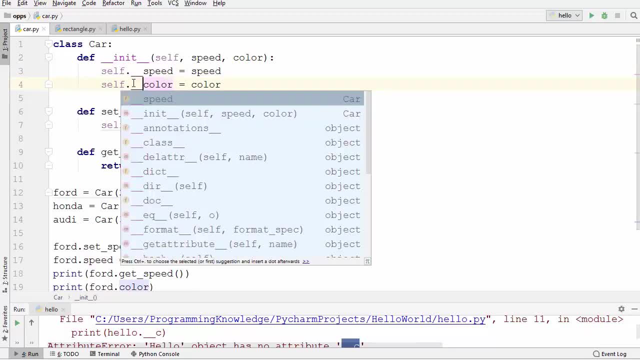 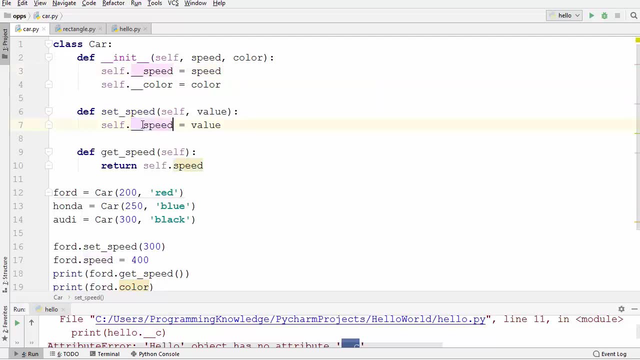 in front of speed and also let's add double underscore in front of this color variable to make both of them private. so I'm going to change this value of speed to in getter and setter also, and now let's try to access this value using this forward object which is underscore, underscore speed. now let's try to run. 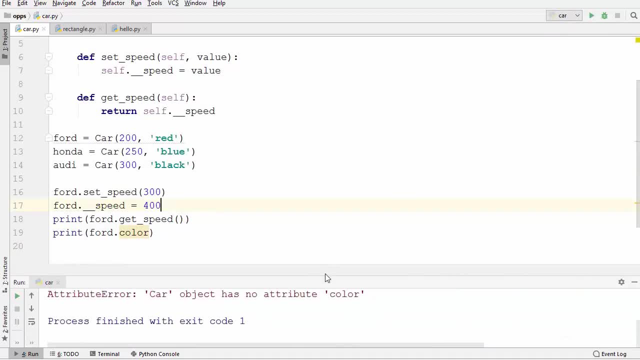 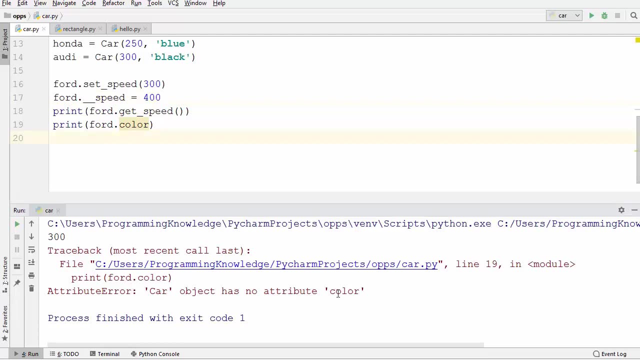 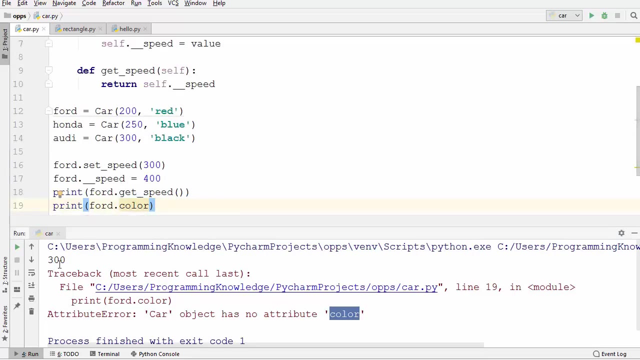 our program. so I'm going to change the file and then run our program and you will see that it's going to give us an error and this error says the car object has no attribute called color, because this variable color is private. now also, you will observe that the value of 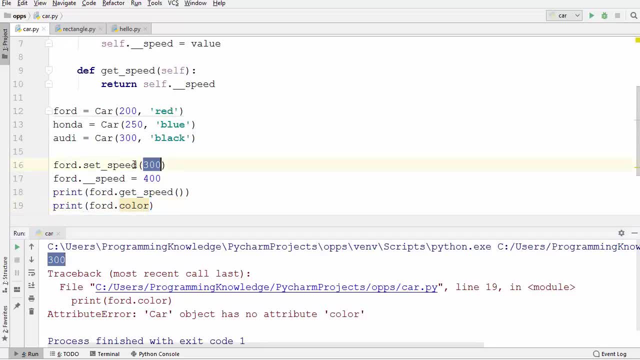 well, the speed is 300, which is set by this set function, even though we have set the speed again to 400 using this underscore underscore speed. but this speed is not changed right. so we cannot change the speed using this underscore underscore variable, because now it's a private variable and that means we cannot change. 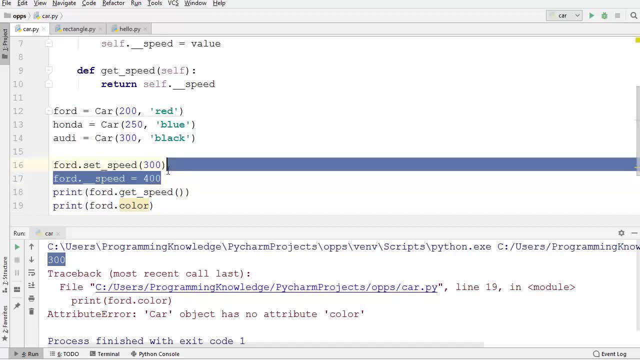 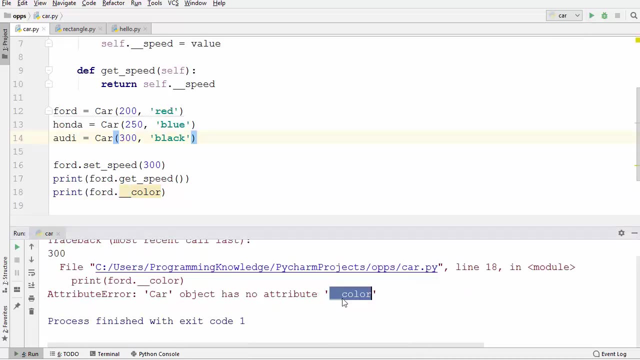 the value using this variable. we need to use this set function in order to change the value of the speed. also, if you want to use this underscore- underscore color here and let's run the code, this will also give you an error because this underscore- underscore color is private. so either you can remove this code or 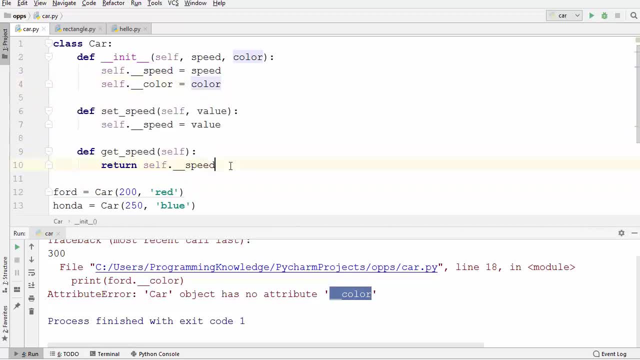 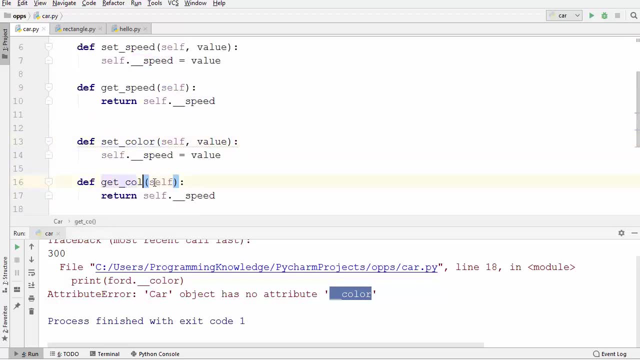 you can create the setter and get a method for the color also. so let's create the setter and get a method for the color. and now we can access the value of color using the get color method, right? so instead of this get speed, we can just write 4 dot get color and it's going to. 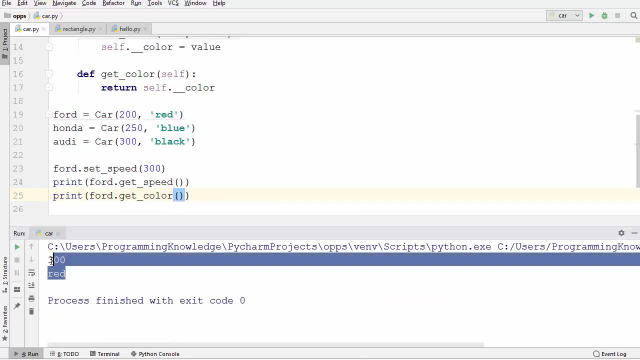 give us the value of color, and now you can see that there is no error and the speed here is 300, which we have set using this set speed method, and color is red, which is the color we have given using this argument in the constructor. and this type of restricting your data access using functions is called. 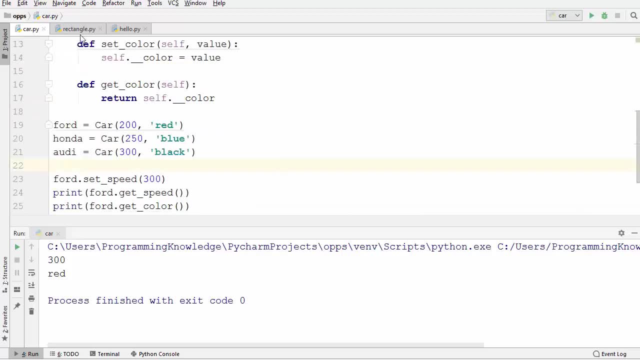 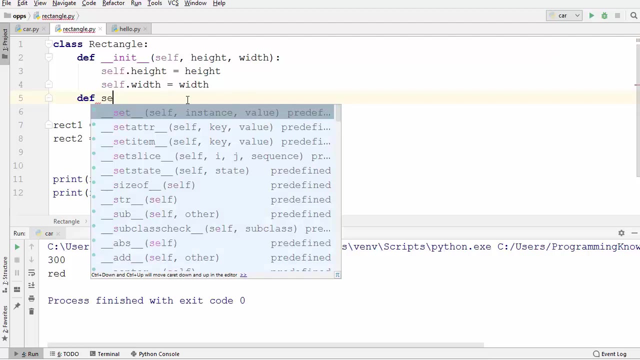 encapsulation. let's do the same thing with our Rectangle class also and let's create the setter and get a method inside the rectangle class. so you already know, we can use this define and then we can first of all set. for example, We'll set the height first of all. 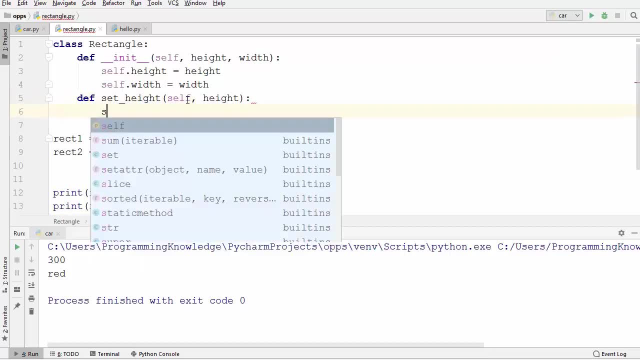 and then we can give the value of height here, and then selfheight is equal to height. right, And don't forget, you need to give double underscore in front of your attributes in order to make them private. So I'm going to do just that. 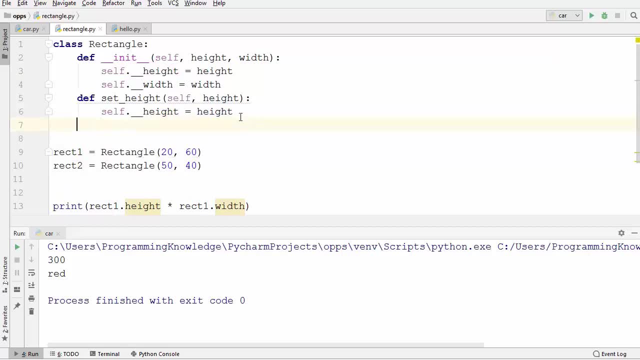 and let's create the getHeight method also. So now we have created the setter and getter for the height, and let's do the same for the width also. So now you have made the height and width as private and we have created setter and getter. 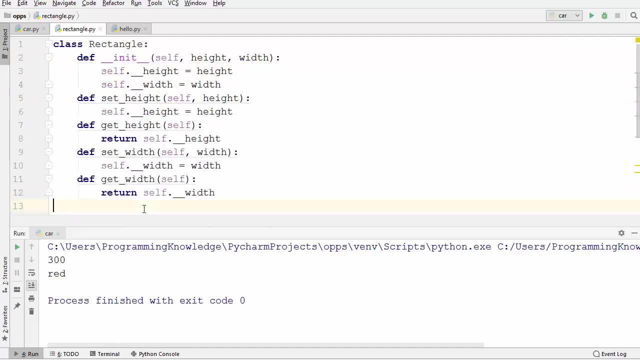 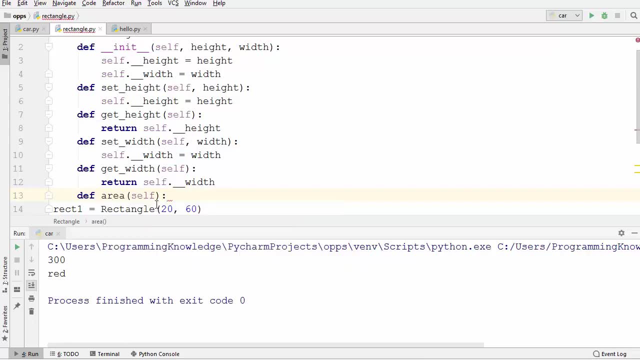 for the height and width. and now, in order to calculate the area, we can define one more method here, which is the area method. So let's create the area method here, and this area method is not going to take any argument, we are just going to return. 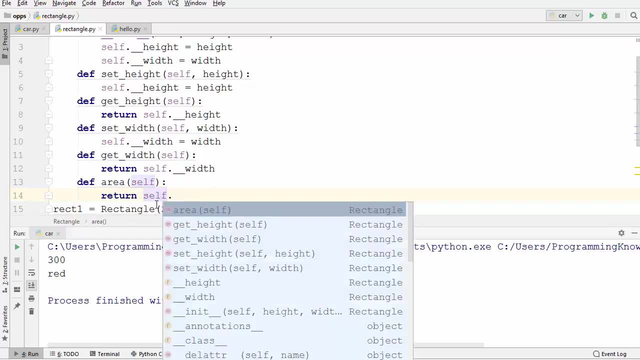 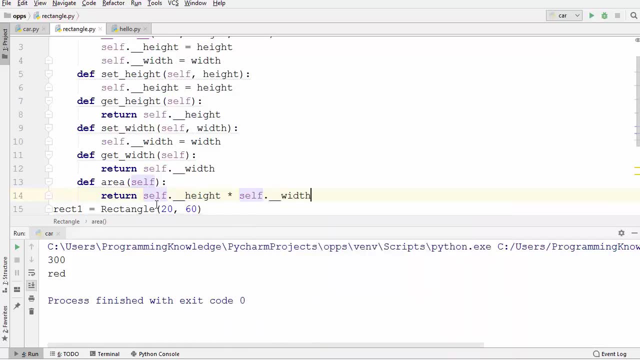 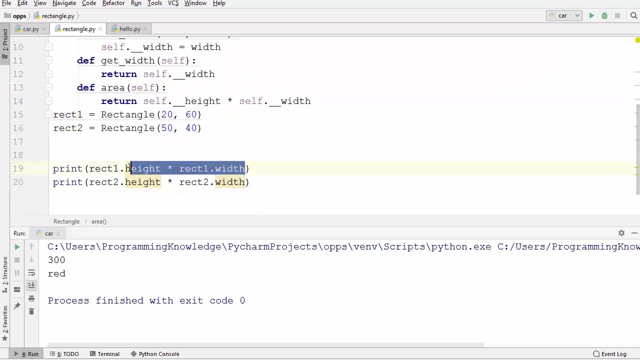 the multiplication of the height, so selfheight multiplied by self__width, okay, Which will give us the area of this rectangle, and we can call this area method instead of using this kind of notation. so rect1.area and rect2.area also. 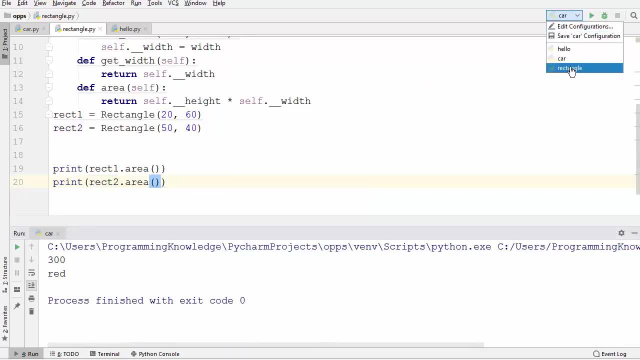 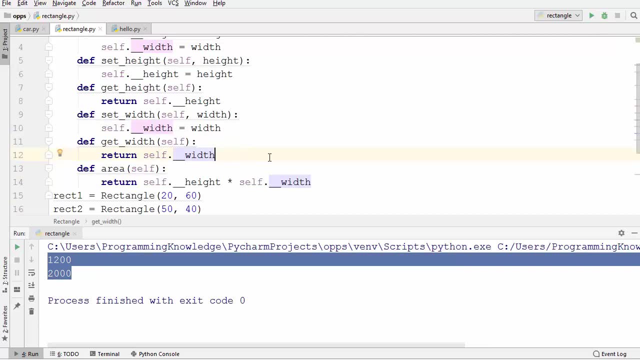 And let's run the code by changing the file name here and run this code and you can see the area is printed now. So this is how you can use encapsulation in Python to hide your data. I hope you have enjoyed this video. I will see you in the next video.